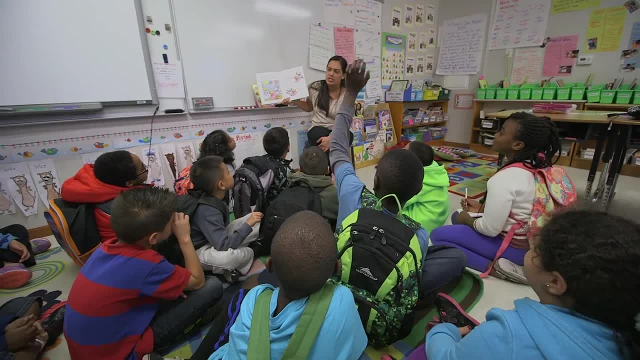 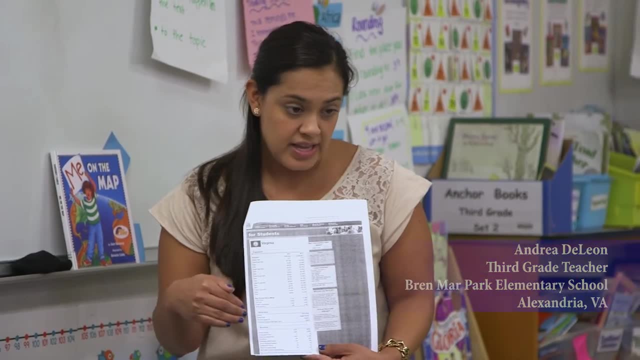 history for geography teachers, but anyone that wants to teach critical thinking skills. The Census Bureau is an organization that goes and they find all this information for us okay And that's what we're using today to answer all of these questions about Virginia. 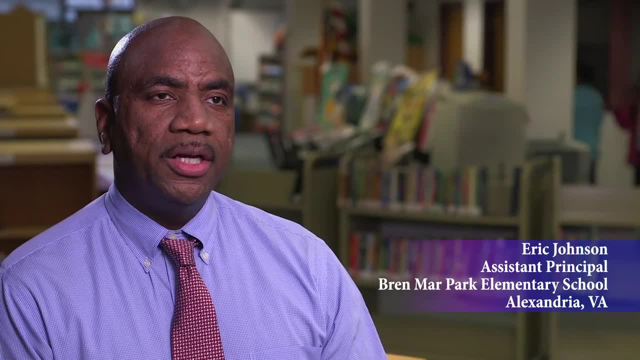 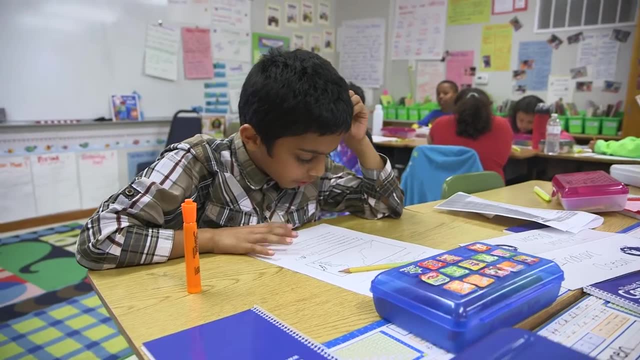 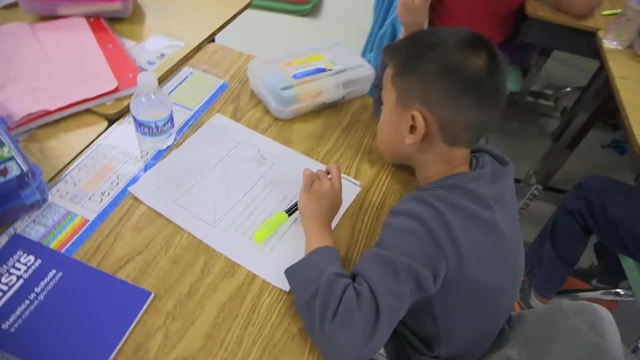 Teachers are the models for the students and I think when teachers show that interest, that vested interest and that passion for bringing the statistics into the classroom, it's definitely going to benefit the students. Students will therefore have opportunities to apply the statistics lessons in many different ways in the classrooms. 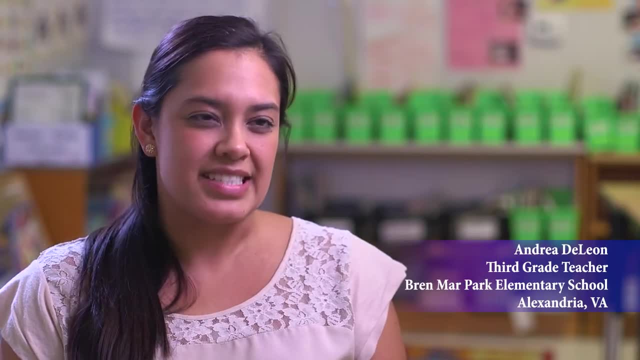 The statistics in school lesson that I did today provided a lot of interesting data, sort of like you know. the statistics in school lesson that I did today provided a lot of interesting data, sort of like. you know, the number of ice cream shops, the. 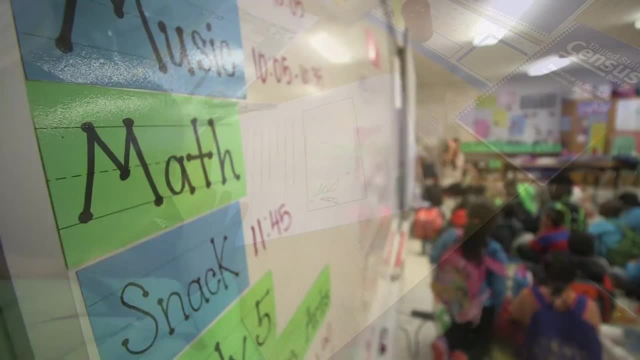 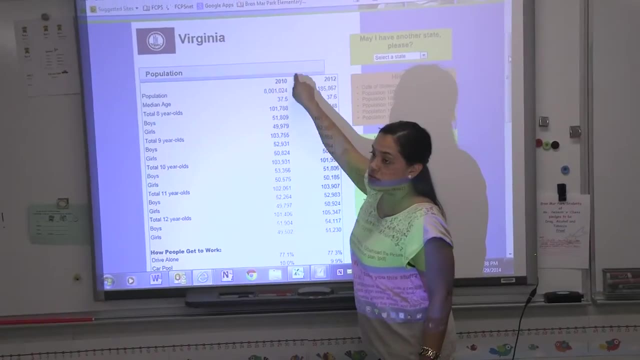 number of dentists in the state of Virginia things that might pique their interest and sort of also make it more accessible to them if they can relate to it. It can be sort of insurmountable if it isn't broken down and I think a lot of children when they get older. 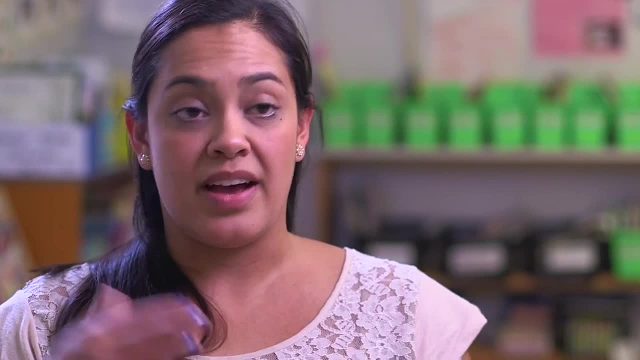 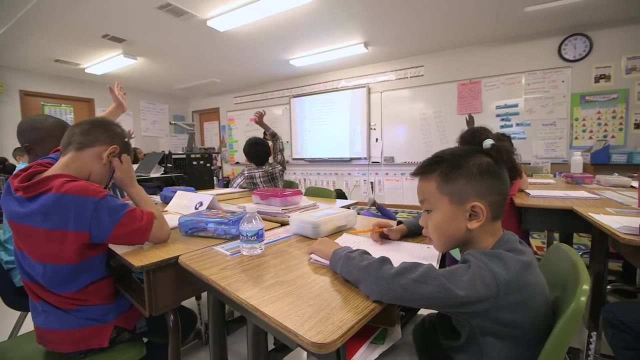 that's almost too late. So if you're starting when they're young and you have activities like this, it prepares them for why it's interesting, why it's important and my goal for them would be, in the future, to be data literate, you know, to perform some of the 20th century. 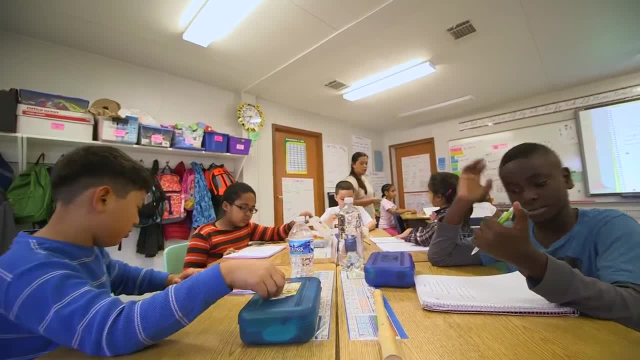 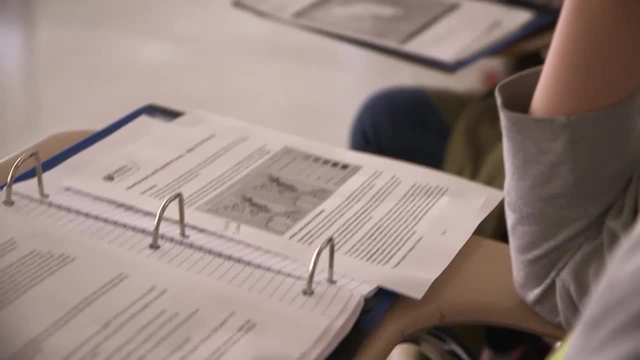 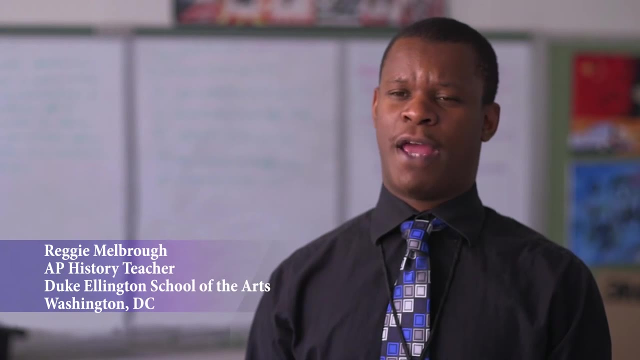 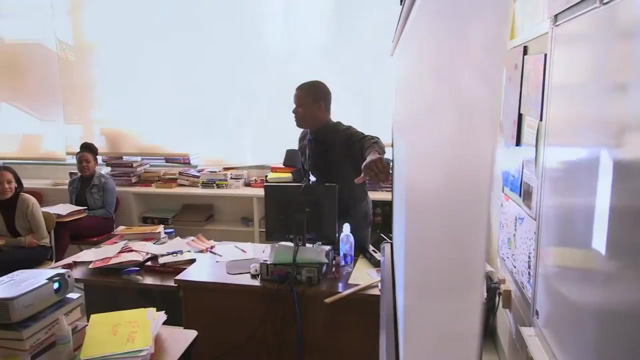 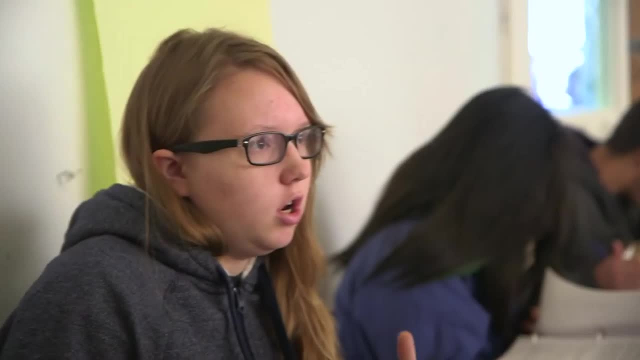 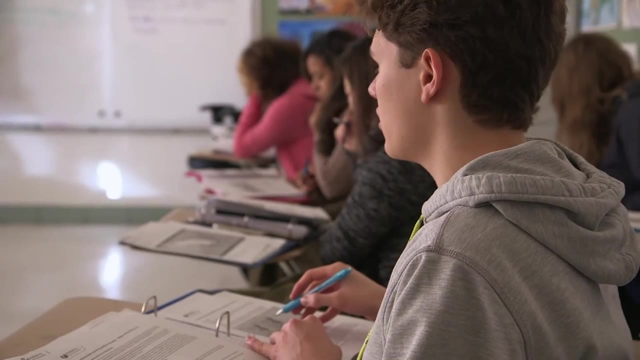 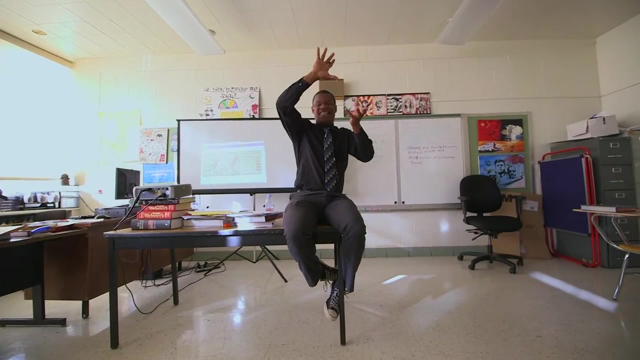 understand what it all means. So to have someone to help guide them to look at the data- not necessarily to say they have to agree with our interpretations, but to at least look at it and determine it on their own- is a good foundation. I think looking at statistics can be kind of mind blowing, but also when you really